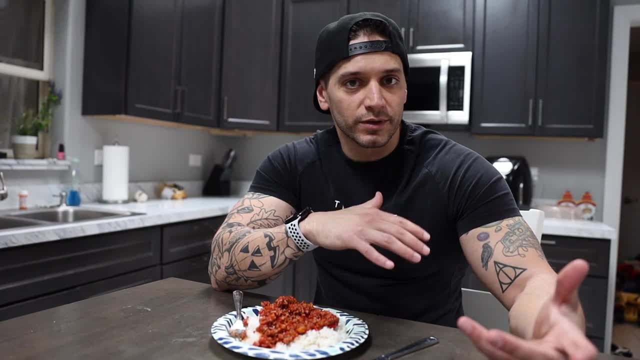 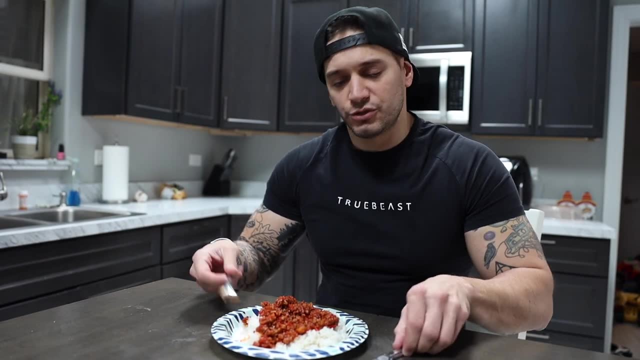 especially when I talk with people that are potential clients or just people that are just starting out in the fitness industry, Just people at the gym that for most people, food in general- like this- is a difficult concept to comprehend. See, for the average person. I feel like when they hear terms like macro counting or 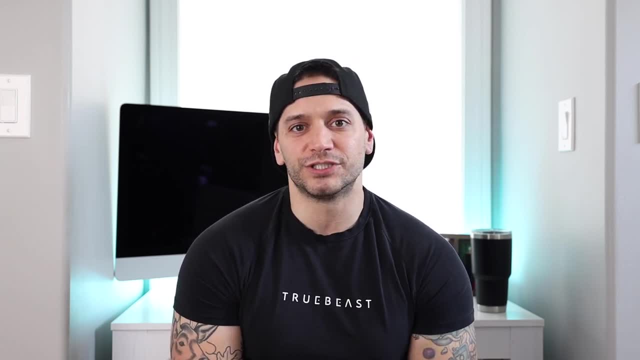 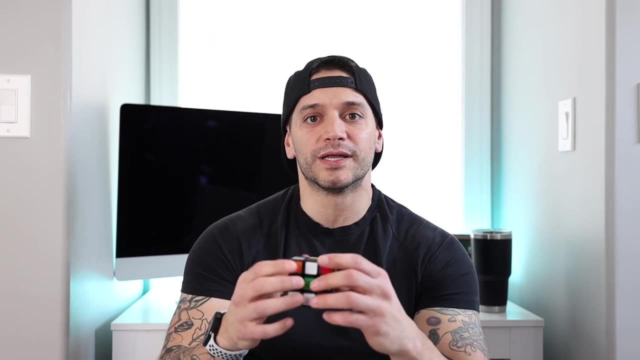 setting calories being in a calorie deficit, total daily energy expenditure. it's something they look at kind of like this: You see it's complex and it looks complicated, but they've seen people do this before and they think that's something that I can do. They try their hand at it. 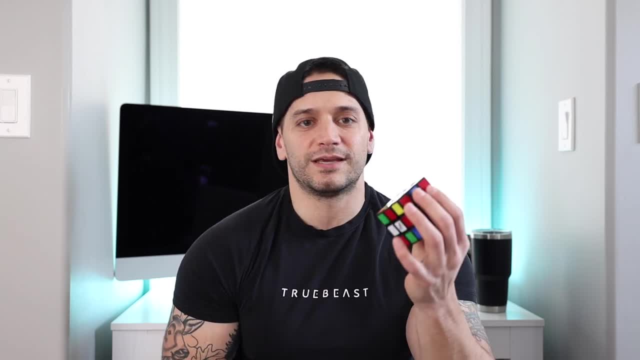 for a while, but eventually they don't know how to do it. They don't know how to do it, They don't know how to do it. They just they get frustrated with it and they give up, which is almost always why they fall off their programming, because they can't seem to figure it out. But for a person like 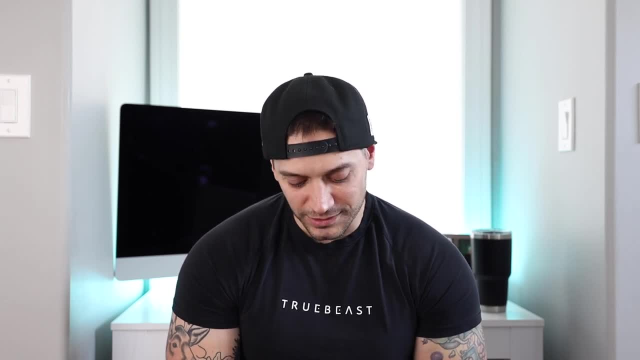 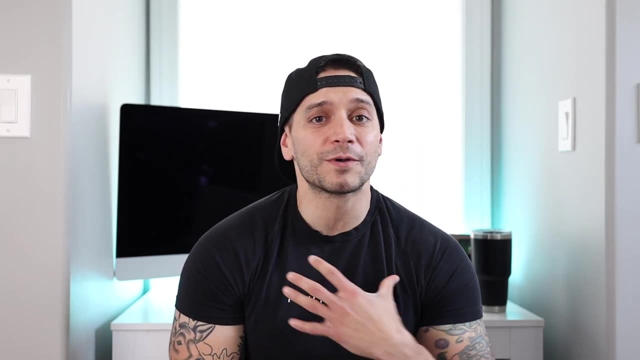 myself, who's been in the gym for over 10 years and have built the discipline and patience we're able to figure it out. So today I'm going to give you a couple of tips on how I'm currently setting up my macros and my programming, and how my calories are reflected in those macros. So 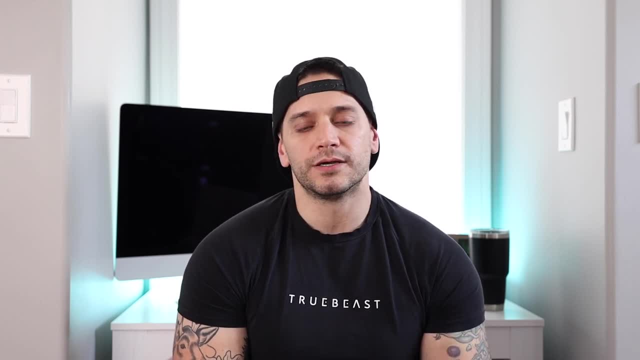 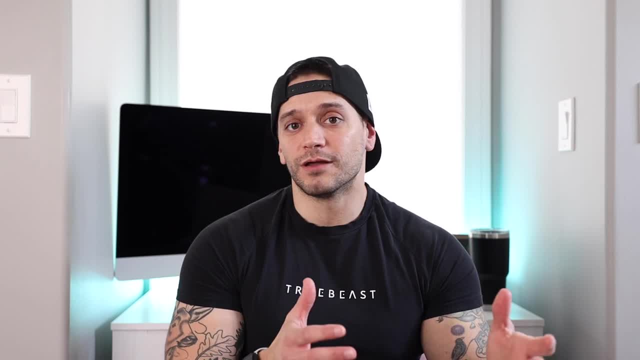 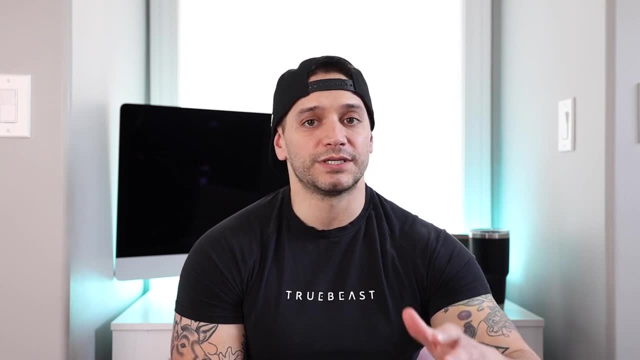 metabolize food differently than the next person, Whether you're using the numbers that I provide today, or if you're working with a personal trainer, or if you're using an app on your phone to try to set macros and count calories. those are really just equations and formulas to help. 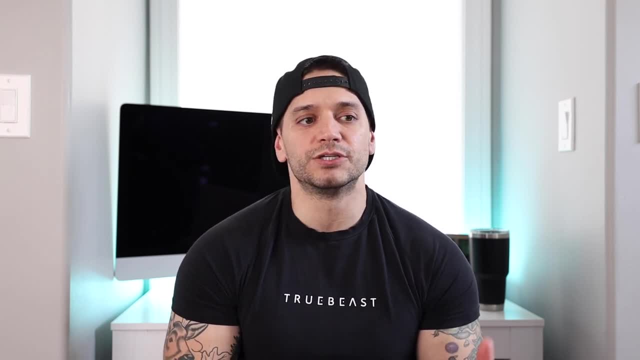 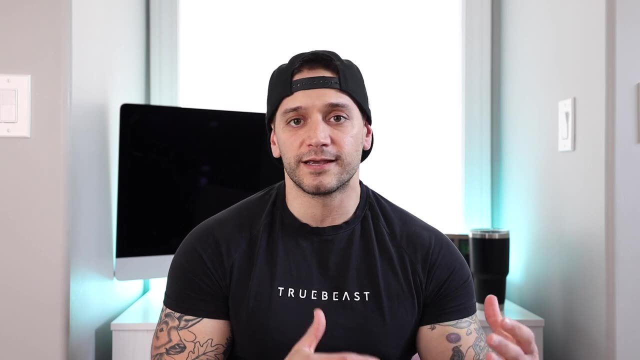 you set a baseline And once you set that baseline, you're going to have to make adjustments as you go. No formula is perfect And it's really important to understand that Now, when it comes to counting calories and setting up macros, it's important to understand that. 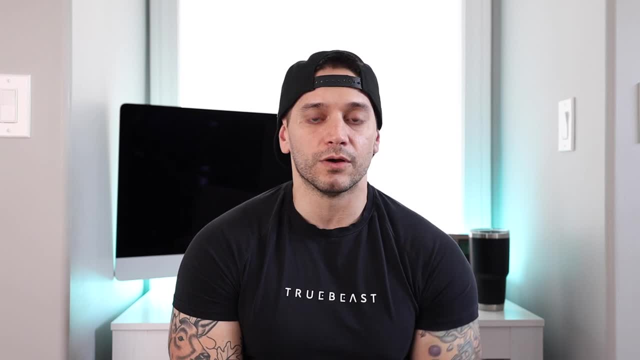 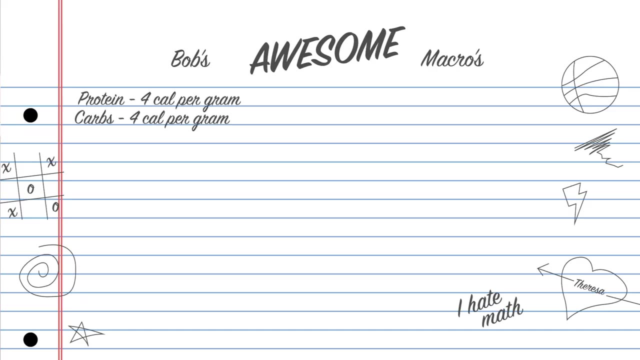 you're going to have to be able to calculate the calories that you're going to get per macros. The most common macros that we track are carbohydrates, protein and fat. Protein and carbohydrates are both going to give you roughly four calories per gram, Meaning if I eat one gram. 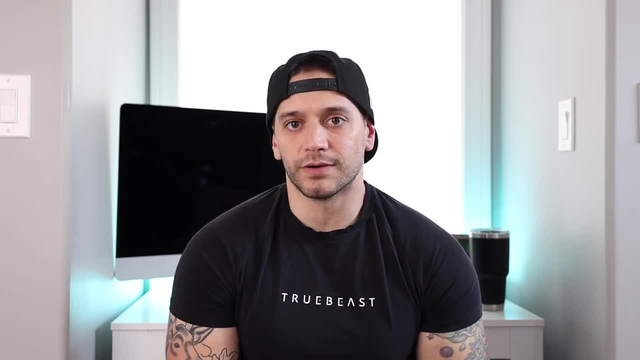 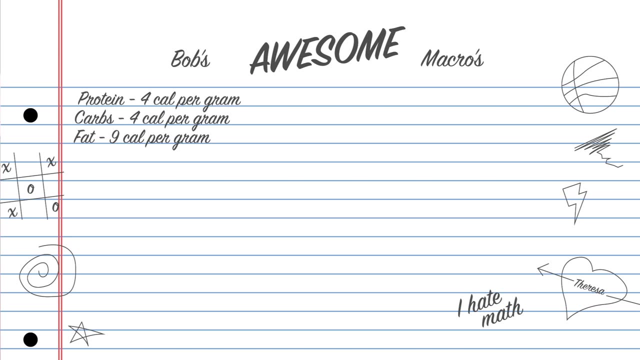 of protein, I'm going to get roughly four calories. And that's the same thing with carbohydrates: If I eat one gram of carbohydrates, I'm going to get roughly four calories. The difference is fat. Fat is such a dense compound It's roughly nine calories per gram, So more than carbohydrates. and 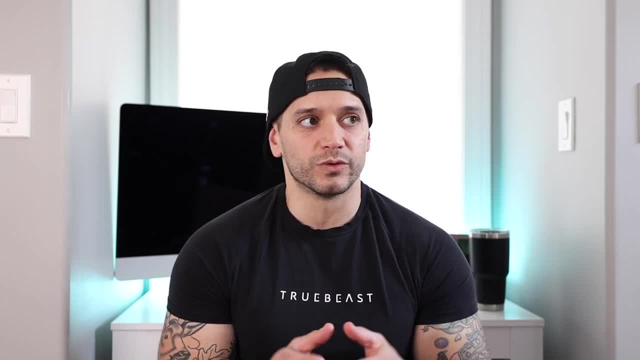 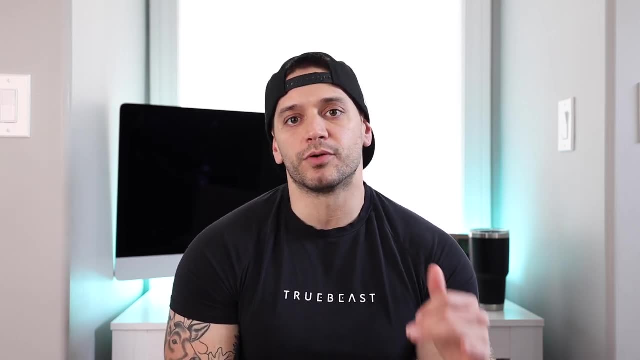 protein combined. Once you have those numbers figured out, it's really just taking those numbers and applying simple math to figure out your numbers. When it comes to my programming, I often set my protein number first. For my body I prefer a higher protein diet roughly. 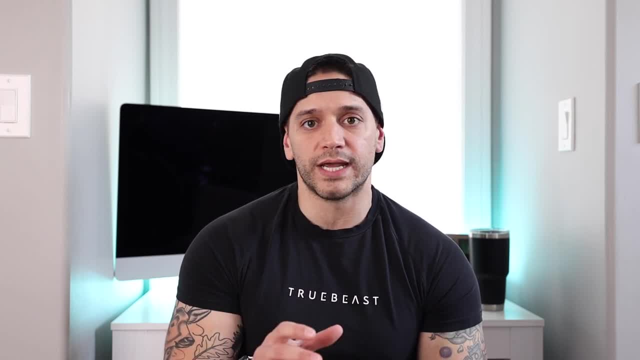 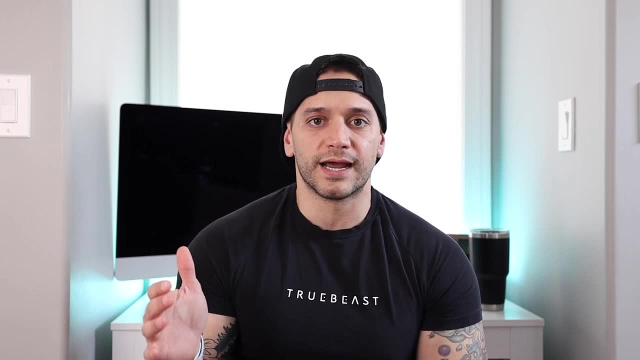 anywhere from 80 to 100% of my total body weight in grams of protein. And to figure out that number right now I'm about 185 pounds. I'll just round up, make it a nice 190 pounds, And I'm always going to err on the high side of setting that number. So what I'm going. 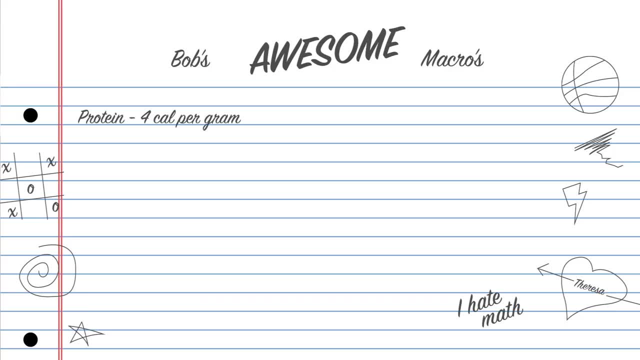 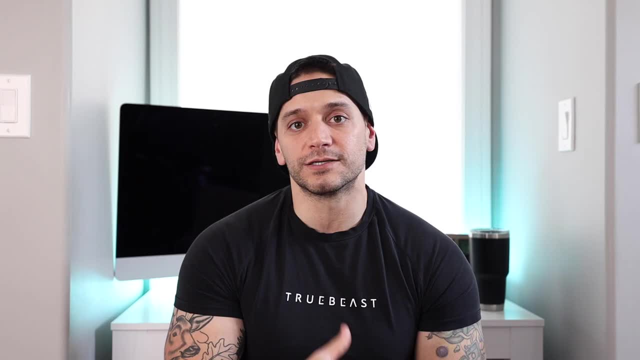 to do in order to set my calories per macro. I'm going to take 190 and multiply that by four and that's going to give me 760 total calories that I'm going to take in every single day for my protein. And just like that, a third of my macros have been set for the day. 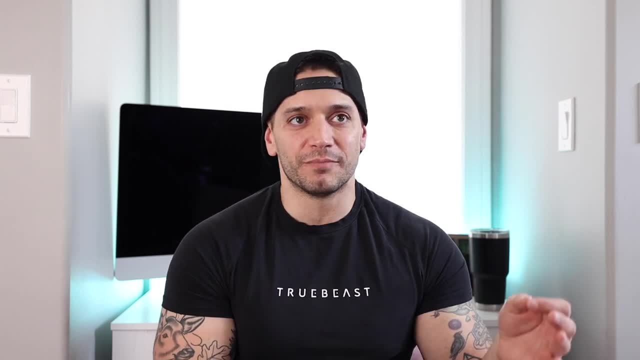 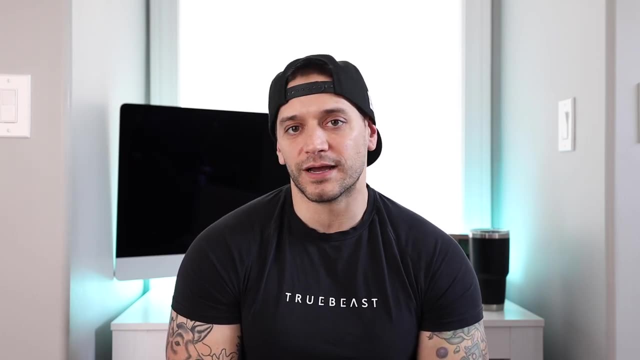 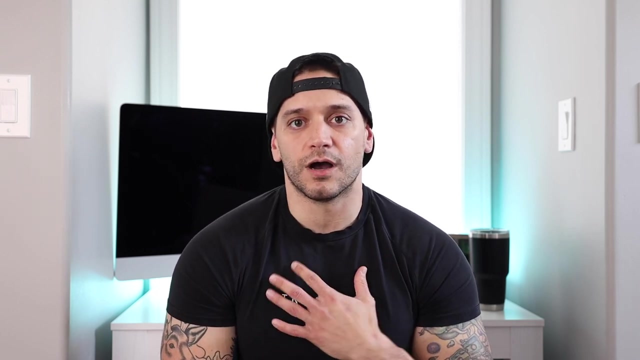 Now the next number that I like to set is my fat, And this is even easier math than the protein numbers, because we know that fat is nine calories per gram. Me personally, I like setting my fat around a hundred grams, So I'm going to set between 40 to 70 grams total per day. I just prefer a hundred grams. 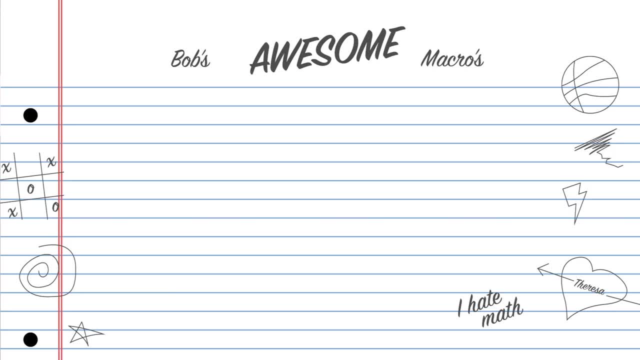 My body functions best off of that number And I try not to go higher than that because, again, it's simple math. Take nine and just multiply that by a hundred and that's going to give me 900 calories every single day from fat Setting. carbohydrates is going to fill. out the remainder of my calories. It's recommended that anywhere from 40 to 60% of your daily total should come from carbohydrates, And how I get that number for myself specifically is: I'll take my protein and my fat. I'm going to take my protein and my fat. I'm going to 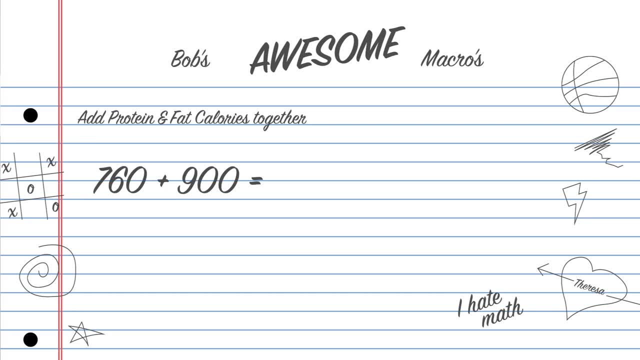 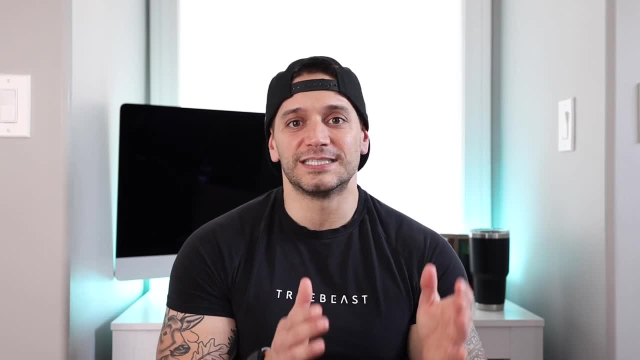 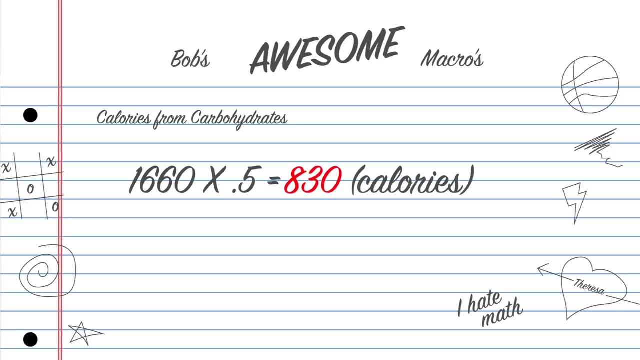 add those numbers together, because I'm going to take 760 and add it to 900 and it's going to give me 1,660 calories. All I'm going to do is take 1,660 calories and multiply that by 0.5 or divide that in half, which is going to give me 830 total calories that I'm going